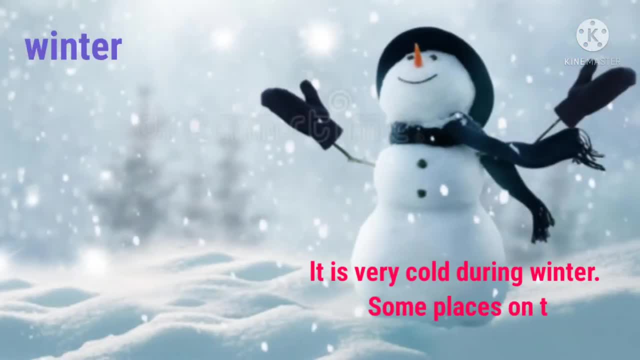 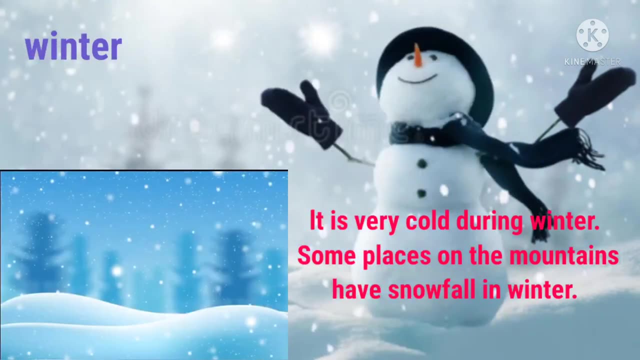 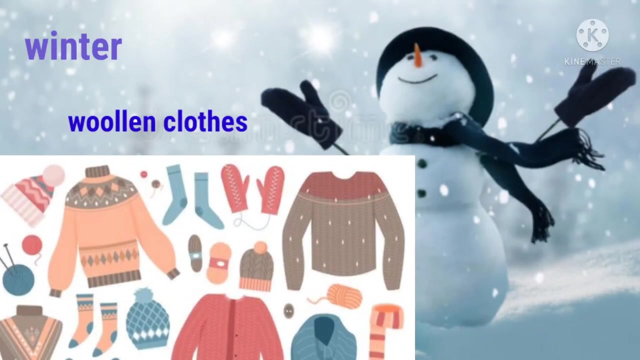 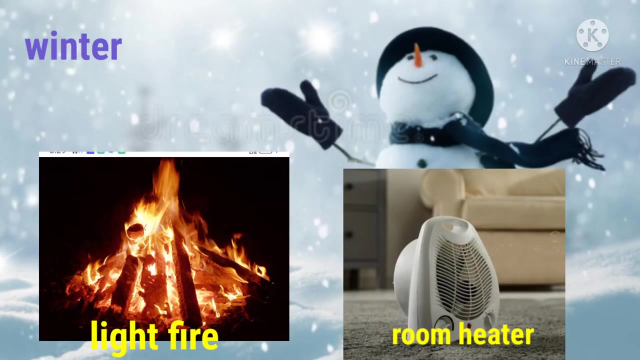 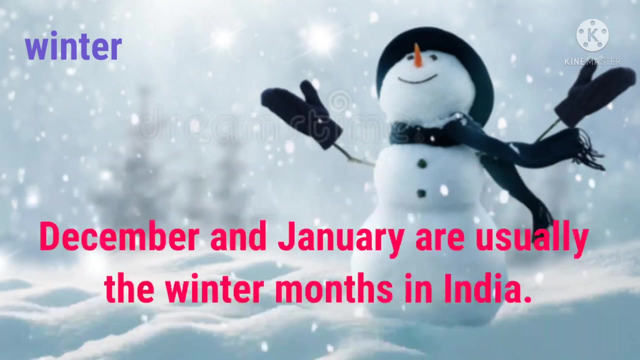 Winter. it is very cold during winter. Some places on the mountains have snowfall. in winter We wear woolen clothes to stay warm in cold weather. We also light fires or use room heaters. We like to have hot food and drinks. December and January are usually the winter months in India. 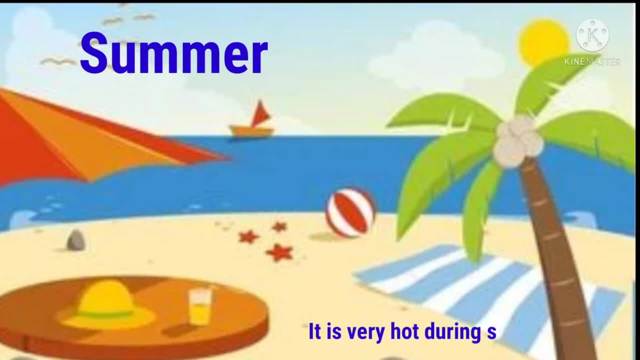 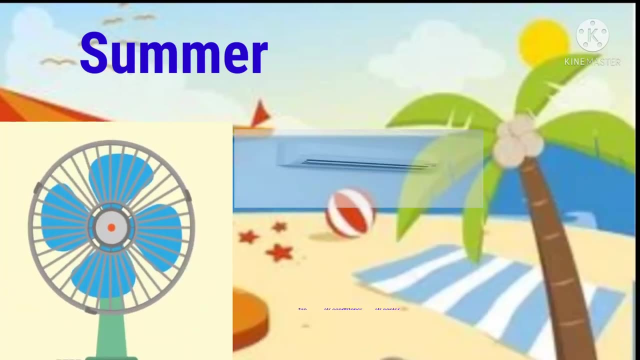 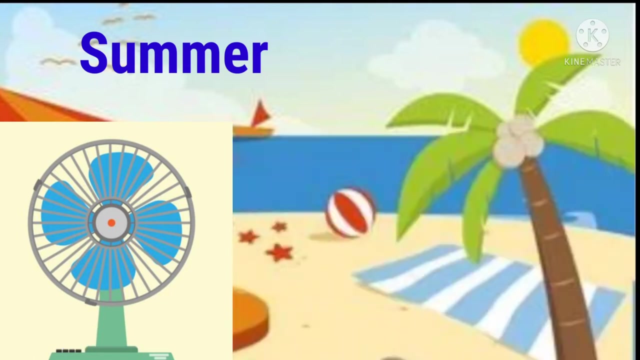 Summer. it is very hot during summer. We wear light cotton clothes. We like to have cold drinks and ice creams. in summer, We use fans, air conditioners and air coolers to stay cool. April, May and June are the summer months in India. 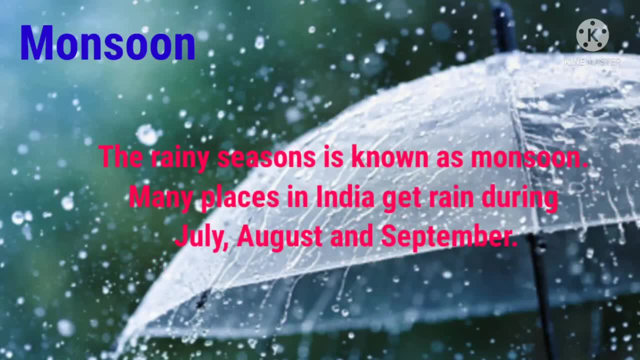 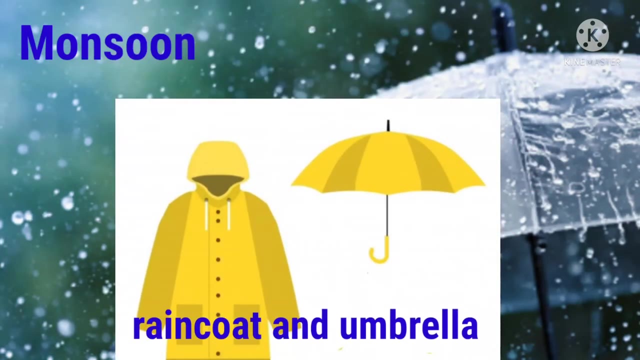 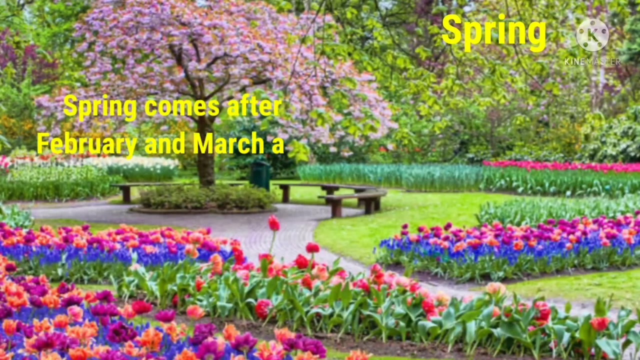 Monsoon. The rainy season is known as monsoon. Many places in India get rain during July, August and September. We wear raincoats or carry umbrellas when we go out in the rain. Spring- Spring- comes after winter and before summer. February and March are the spring months in India. 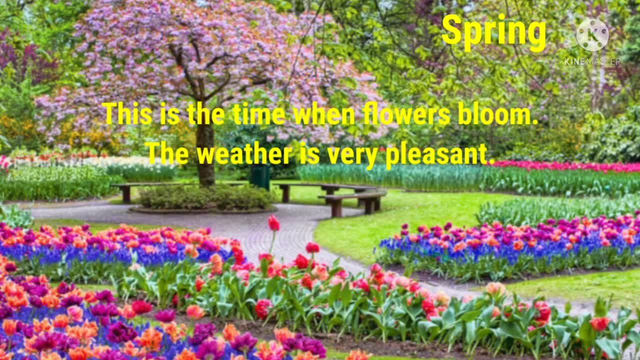 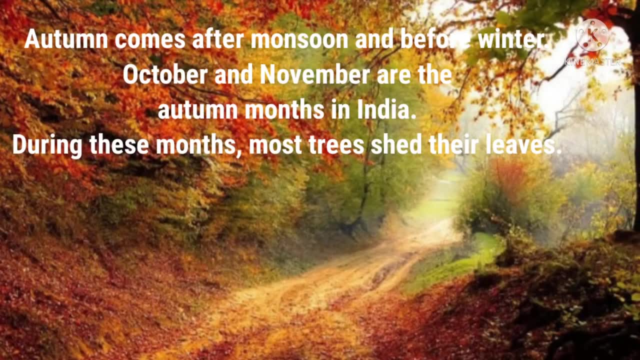 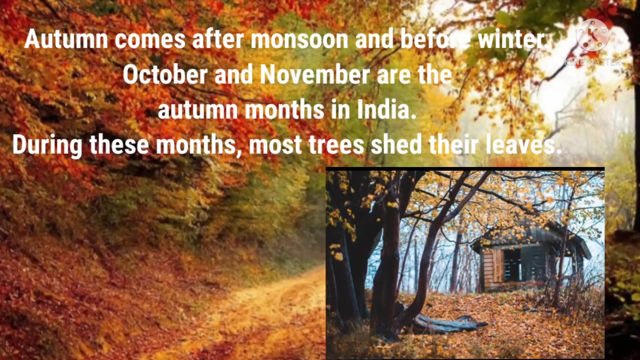 This is the time when flowers bloom, The weather is very pleasant, Autumn. Autumn comes after monsoon and before winter. October and November are the autumn months in India. During these months, most trees shed their leaves. Children, before concluding today's class, let us revise. 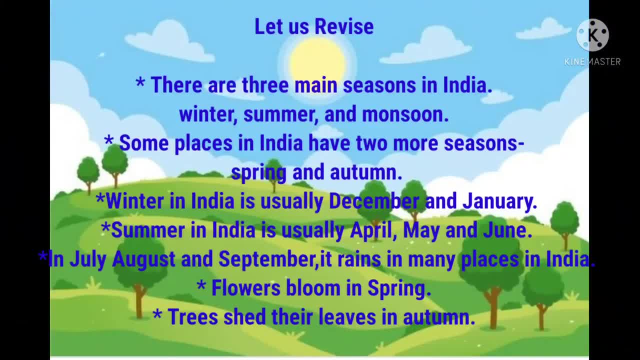 Children. there are three main seasons in India: Winter, Summer and Monsoon. Some places in India have two more seasons: Spring and Autumn. Winter in India is usually December and January. Summer in India is usually April, May and June. In July, August and September it rains in many places in India.